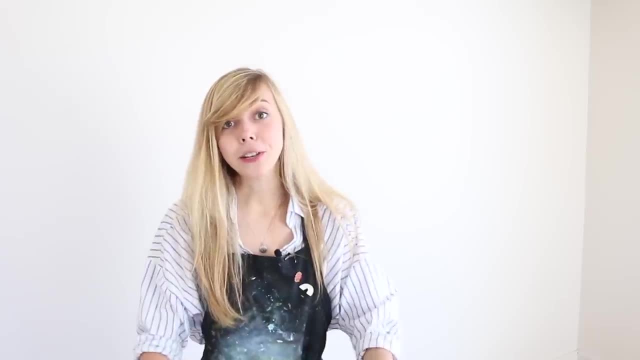 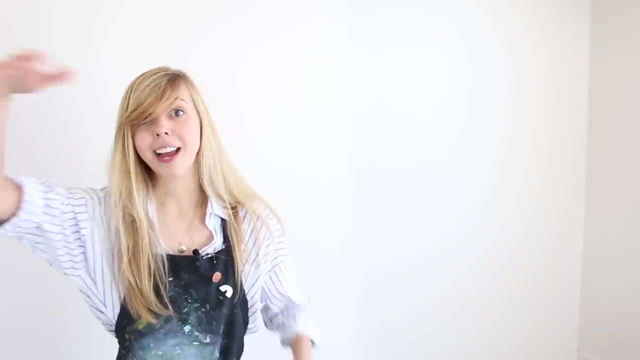 someone. If you've been around for a while, I'm sure you've met. If you are new, this is my very, very special, important friend, my lovely assistant, the apple of my eye, Hoodie Hoodie is going to. 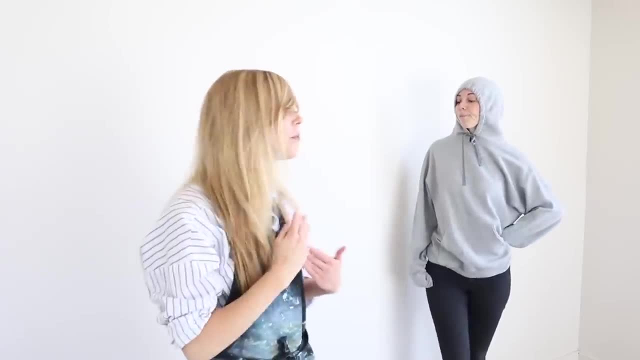 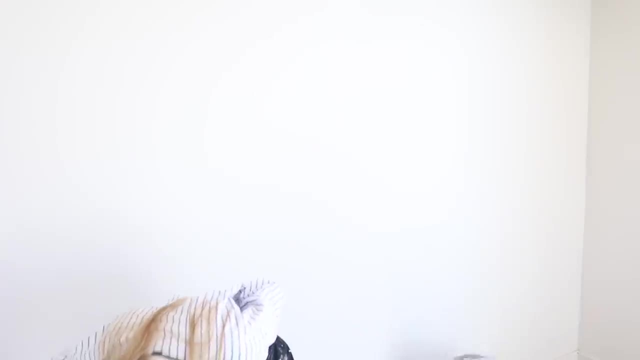 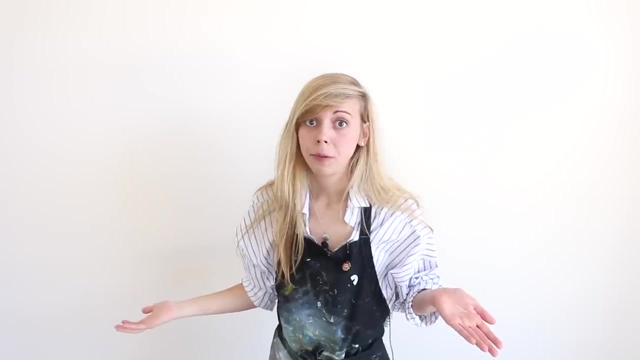 help us demonstrate some very important topics today. so thank you for being here and I hope you guys enjoy this video. Number one – composition. Have you ever made a piece and felt something was just off about it? A lot of times what's wrong has to do with your composition. Composition refers: 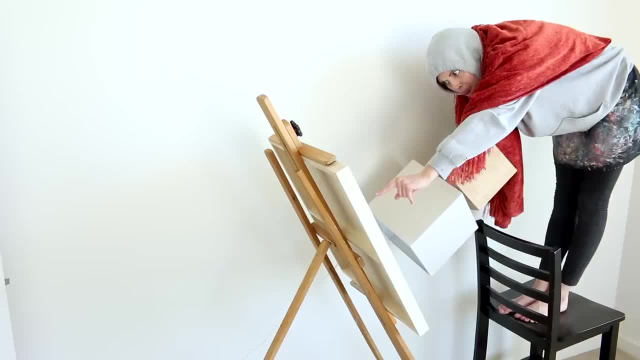 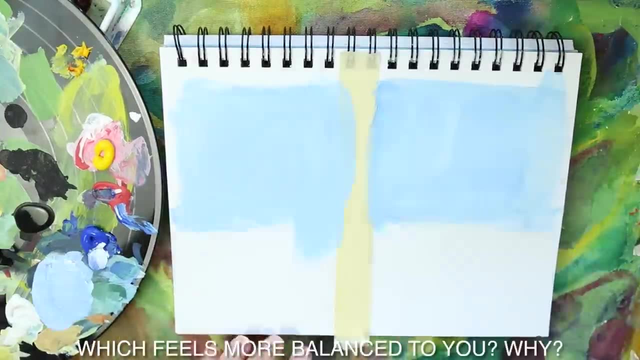 to the placement or arrangement of different visual elements in your artwork. Through your arrangement of colours and shapes, a piece can either feel balanced or imbalanced. It's important to pay attention to where your visual elements in work lead the eye. Do you have? 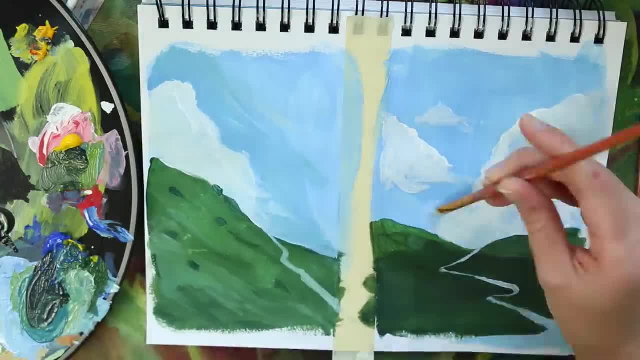 a large or bold element on one side that is not countered by another visual element, Whether there's a detail that really checks in, and if it's something that is really being connected or unsure of or something else that needs to be worse, be careful with it or be careful. 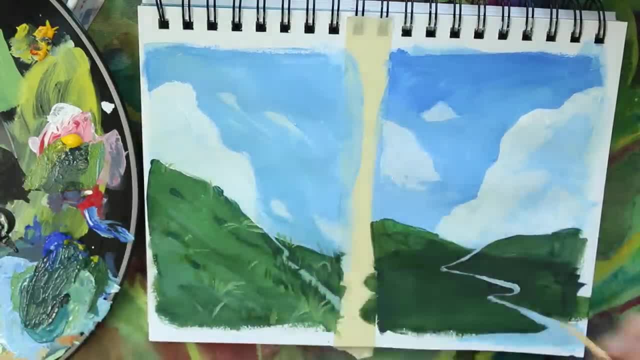 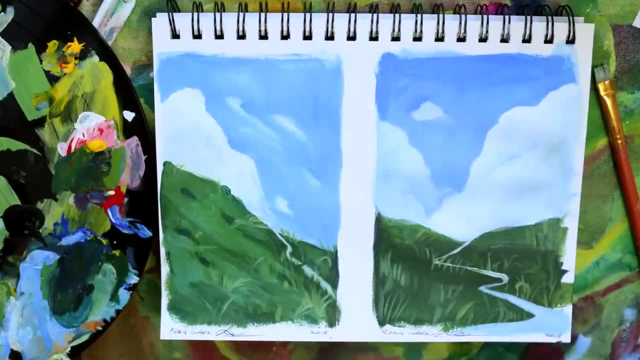 on the other, Or maybe do you have a series of optics creating implied lines that lead the eye off the page. By adding visual balance or elements that circle the eye back around to your image, you can put at ease the awkwardness of a piece masking tape. Do you want to get experimental or loose in your 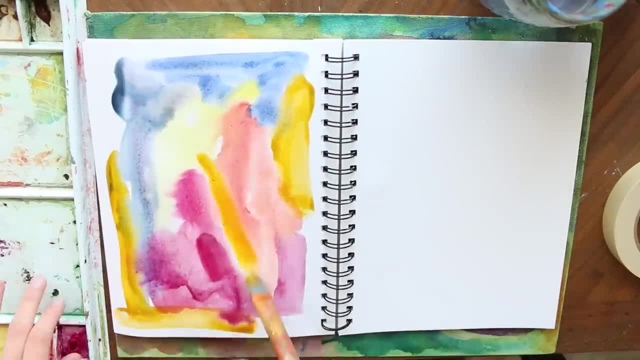 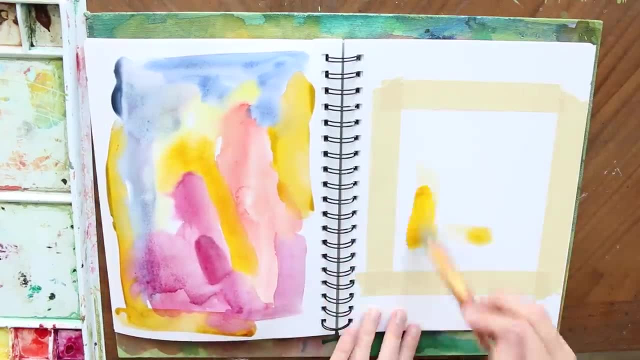 sketchbook. Maybe try something, or practice something you're really not feeling confident in. Try simply adding masking tape. By squaring off the edge of an image in your sketchbook, you can immediately add structure to the work and amplify the overall presentation. Remember this hack, too, though, when you 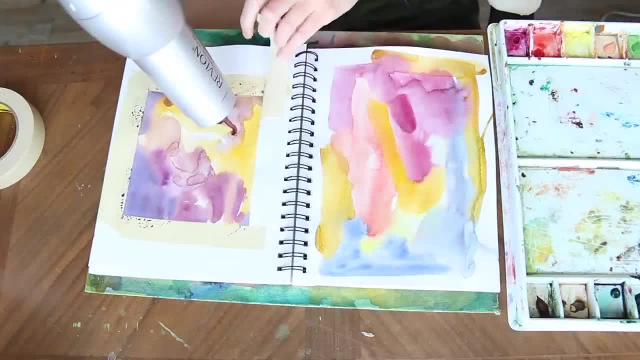 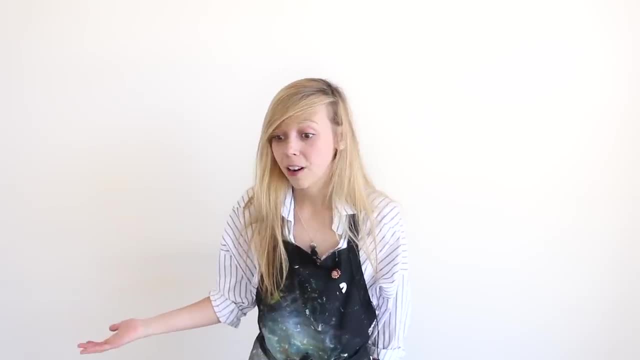 do it Before removing your masking tape. use a hairdryer to create heat to break the adhesive. This will protect your paper from tearing. 3. References: Now that I've been sharing art advice online for a couple of years, this idea has only 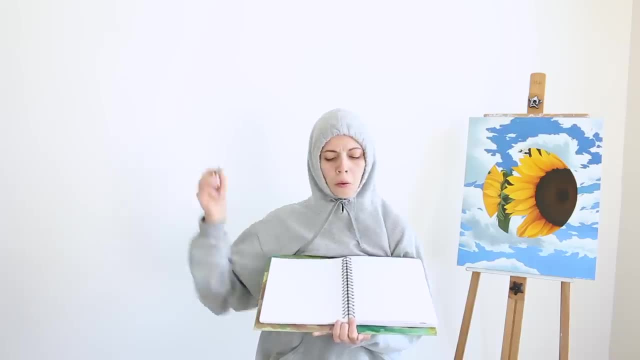 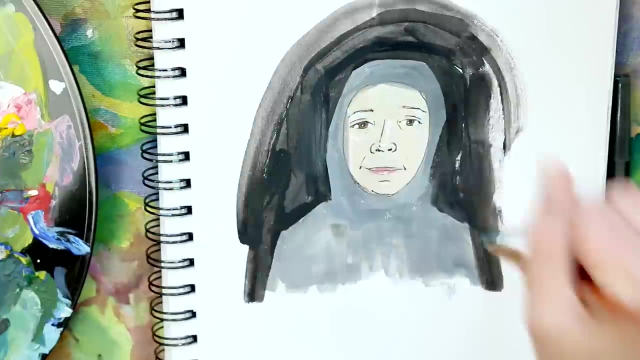 strengthened to me. Have a reference. Whether you're looking at something in life or in a photo, having a visual reference will deeply improve the quality of what you were able to make immediately. Instead of relying on memory or skimping through your sketchbook, start looking at the lyrics of your work right now. 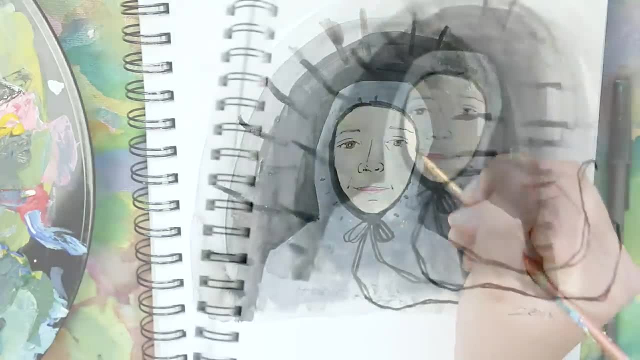 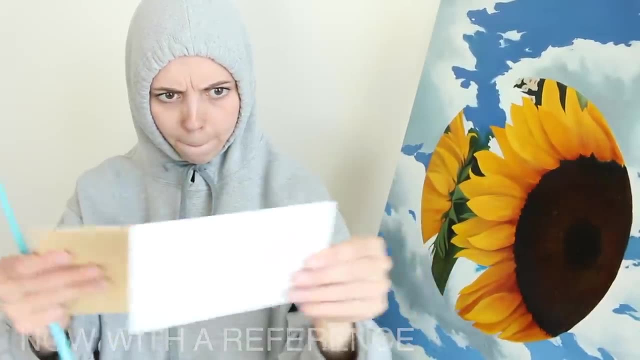 or false perception. you have an increased access to reference for detail, color, perspective, form, anatomy. I've seen time and time again people, within days of each other, make pieces, one from memory or imagination, the other from a good reference, and the difference is startling. 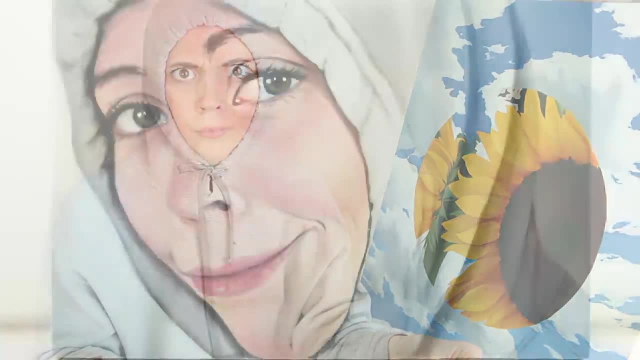 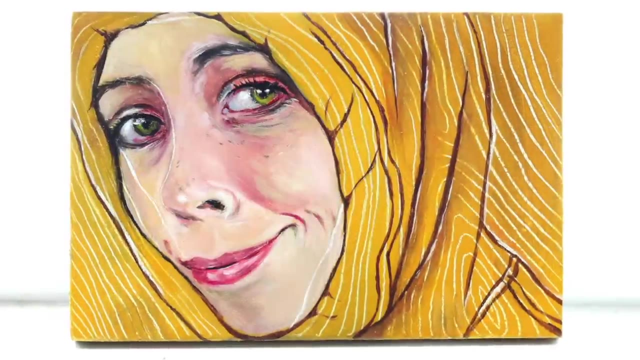 Of course, not everyone wants to work realistically, but often pulling a reference from which you can break stylistically but at least pull visual cues or ideas from, will improve a stylized image. Four transfer drawings: This has been paramount to my personal work. 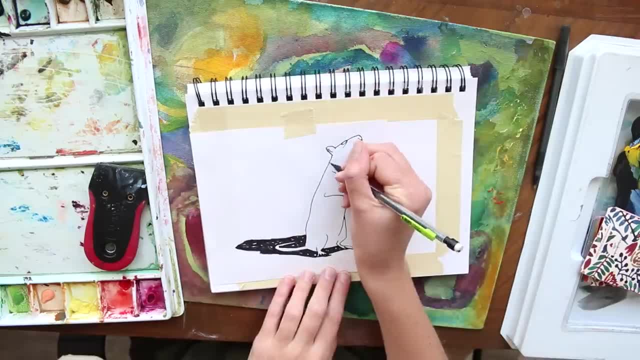 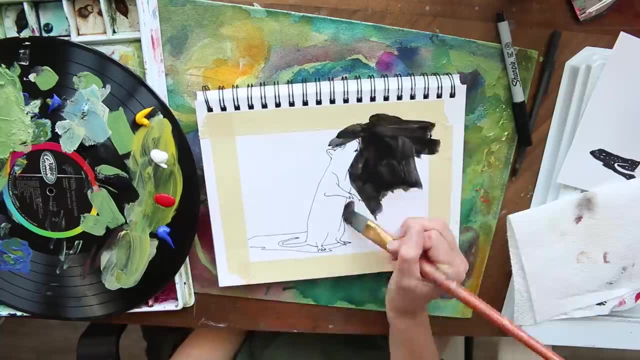 Honestly, it's something that's both improved my art in the short term and the long term. Transferring an image- essentially tracing an image- will give you a solid structural base to work on top of. You can use it to work realistically or as a line guide from which to deviate in more. 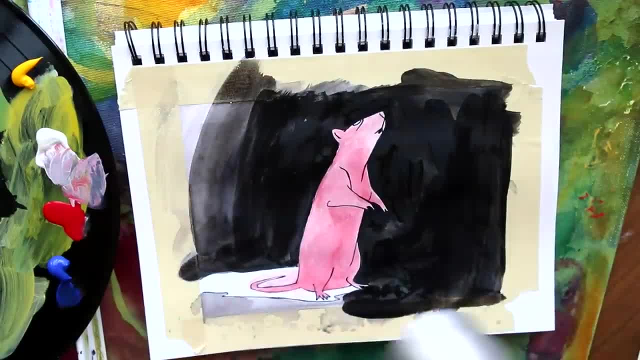 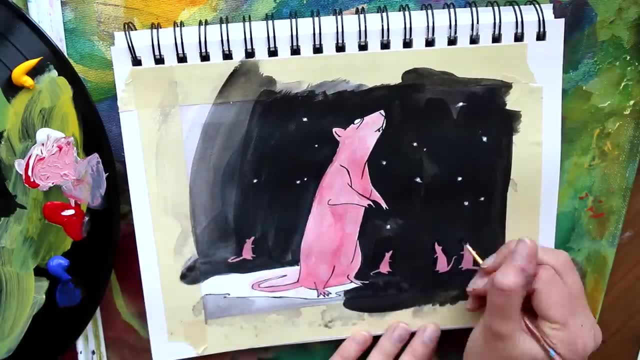 stylistic ways. There's much more to making a good piece of art than being able to draw realistically. Tracing an image will not ensure your art is great. How you fill those lines or accentuate them creatively is up to you, But these guiding lines will largely ease your ability to begin with a strong starting. 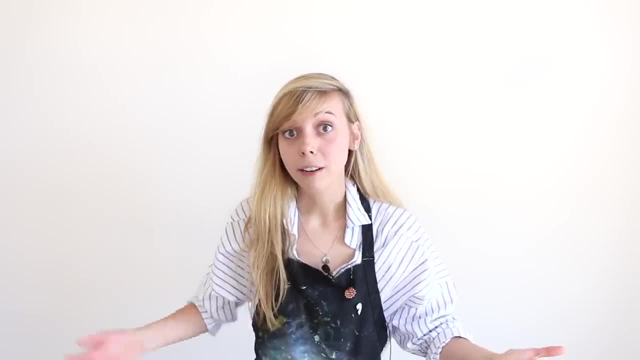 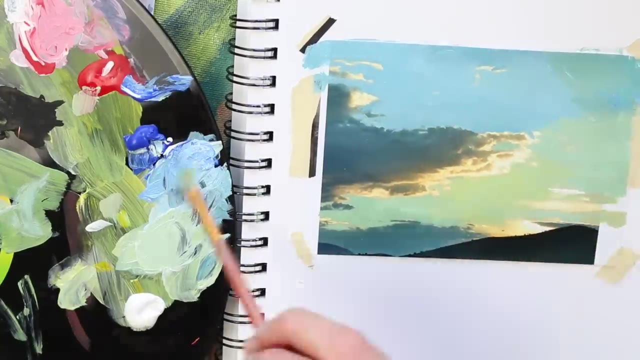 point Five: premix your colors. If you're hoping to achieve very plan-specific colors, perhaps to replicate an image, scene, portrait or design, premixing your colors will help you achieve color accuracy. You can mix them and compare them against the color you are trying to replicate or 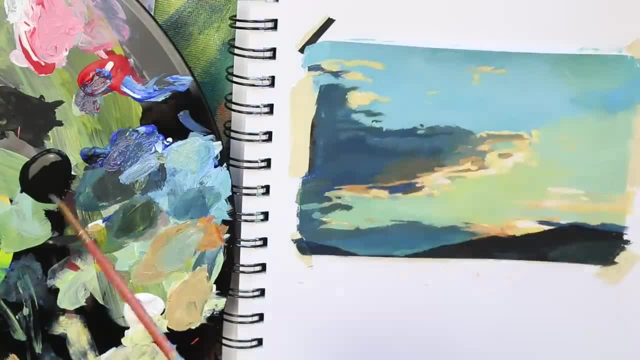 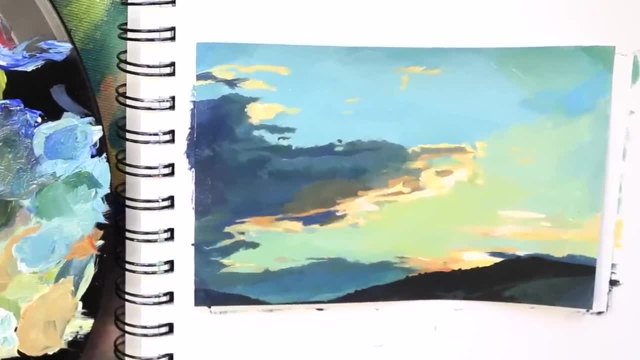 just mix them and find a color you really love before beginning. This will save you from having to paint and repaint Or ultimately settle for colors that weren't your ideal in the first place. Six: use the right surface. What you work on top of matters. 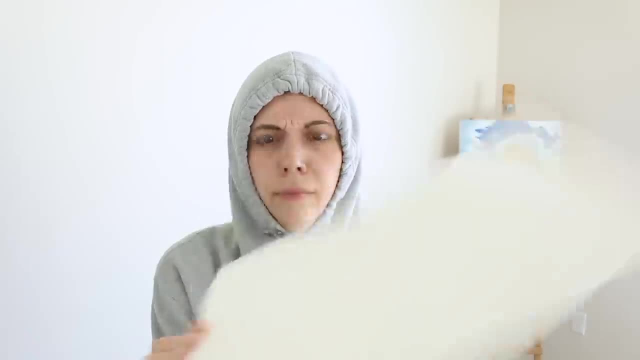 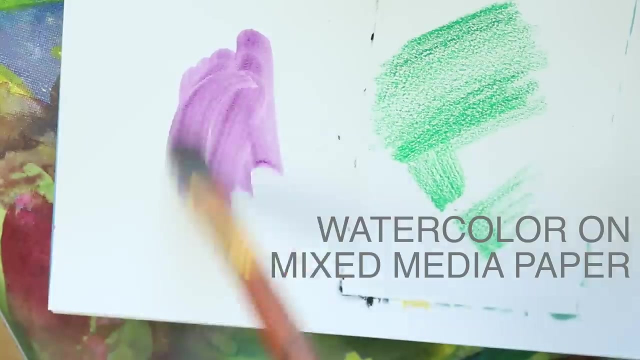 Different paper has different uses. There are variations such as texture, thickness, softness. While one paper might be great for drawing, it could buckle or tear when used with watercolor. Having the right kind of paper will leave your overall work looking much more or less. 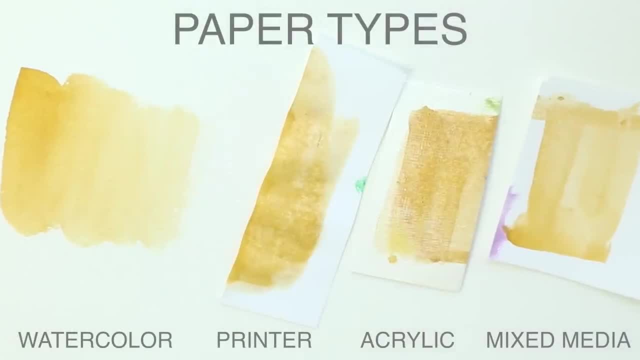 professional and valuable. Same idea applies for drawing. If you have a heavily textured paper and want to shade realistically, you can use the same idea for drawing. If you have a heavily textured paper and want to shade realistically, you can use the same idea for drawing. 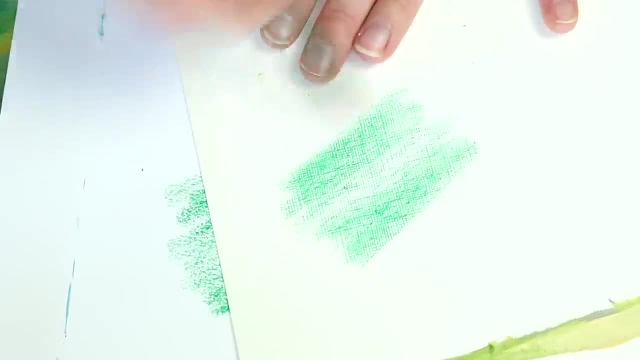 If you have a heavily textured paper and want to shade realistically, you can use the same idea for drawing. Large grains or texture will distract from how smoothly you are able to create shades or contrast Beyond just paper, though. know what you like. 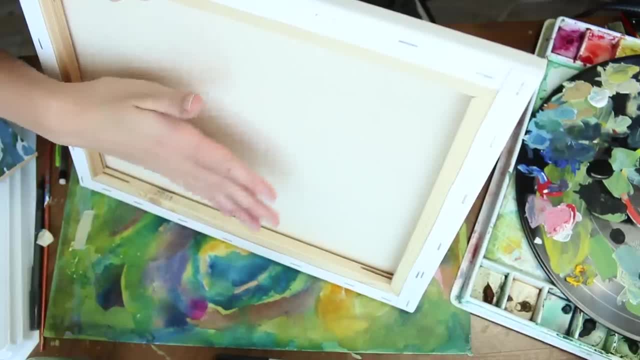 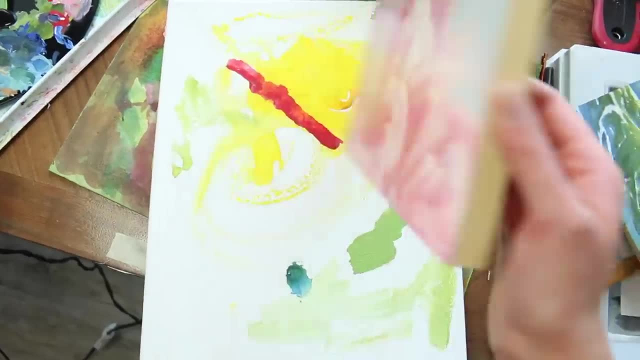 If you're a painter, you may find you love the grain and bounce of a stretched canvas, But you may adversely find how much you prefer to work on a smooth wooden panel. It will play into the kind of image you are able to make and your overall surface texture. 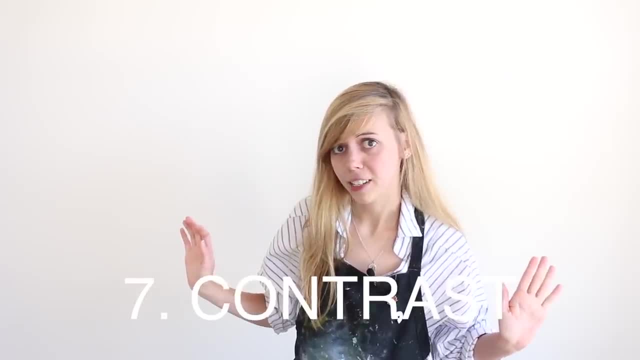 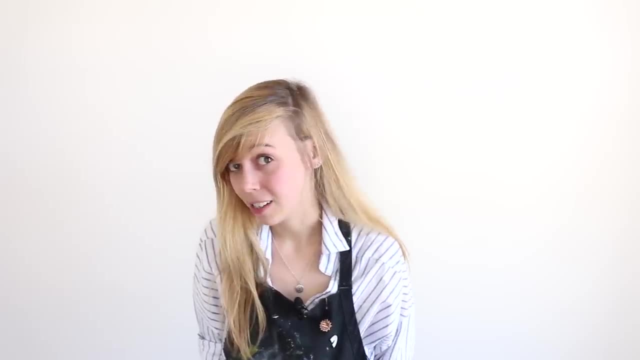 and aesthetic Seven bump up your contrast. Are you paying attention to your highlights, midtones, shadows? Your colours may be different, but are the tints and shades different? If you were to put an image of your work into Photoshop and put it in greyscale, how much? 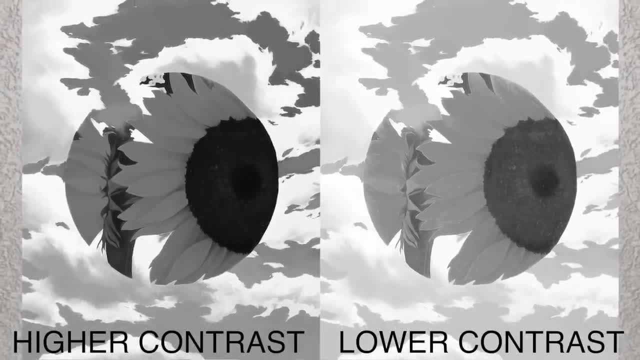 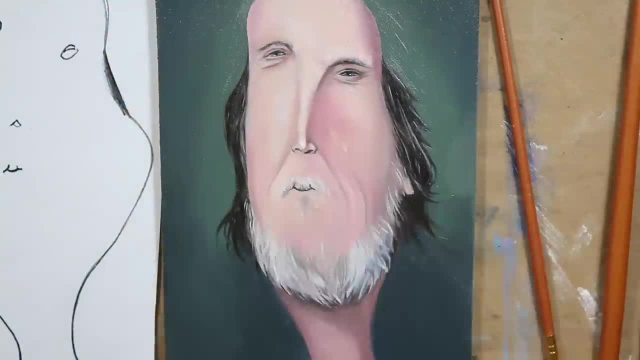 contrast would there be. Having attentiveness to your highlights and shadows increases the depth and visual interest of your work and increases present visual illusions. One tip on how to increase your contrast in oil painting is to do glazing With this. first, let your piece dry. 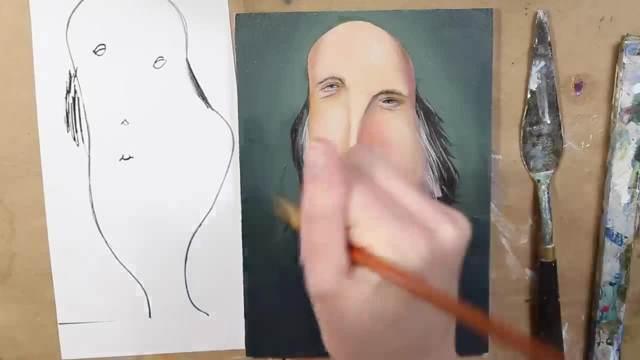 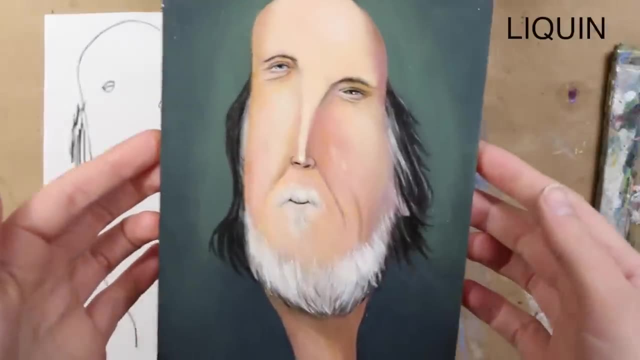 Then you can bump up the saturation, change the hues or add contrast and gloss by mixing a small amount of paint with a decent amount of medium. Here we're using Liquin. This creates a translucent layer of colour which you can use to overlay on your background. 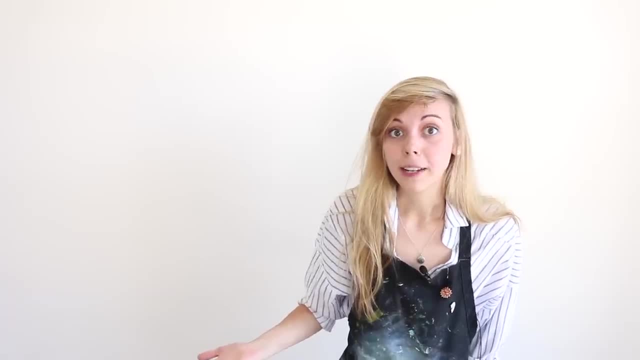 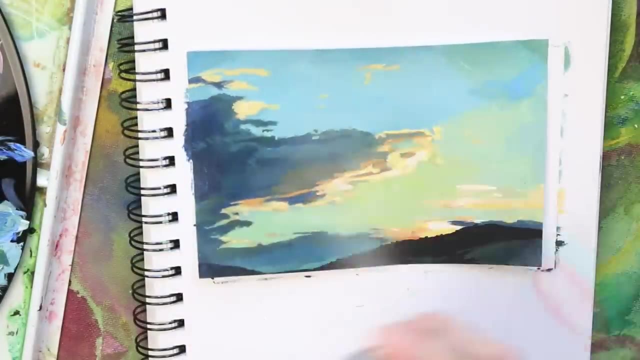 image: Eight varnish. A simple way to elevate your piece is to just use varnish. You can use a pore liquid or spray. This will protect the surface when it dries as well, if desired, give it a glossy appearance. 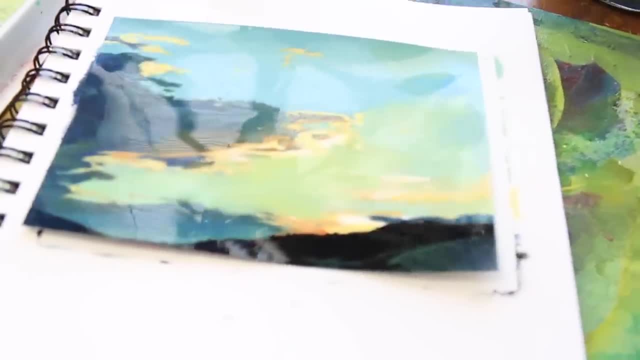 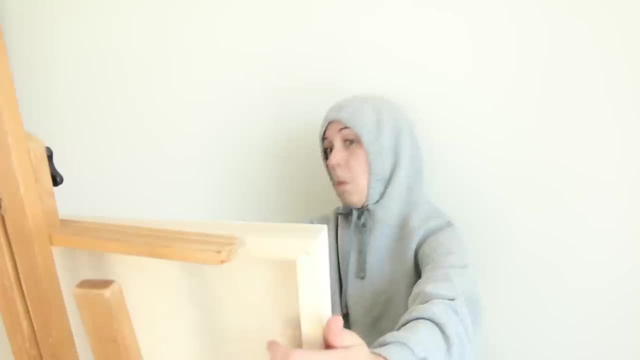 With that simple act, a glossy overlay can immediately give your piece a more polished and vibrant appearance. Nine: get fresh eyes. Often we get so lost in our own work we stop being able to see it objectively and glaringly obvious problems become invisible to us. 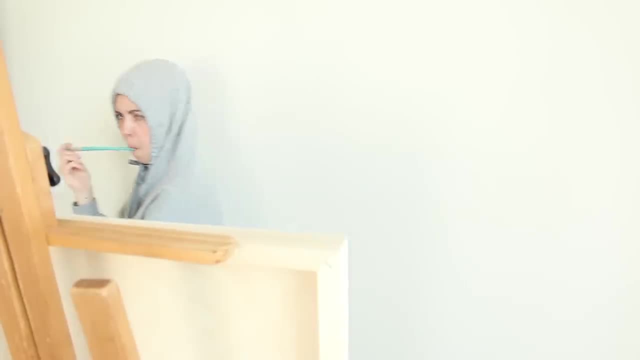 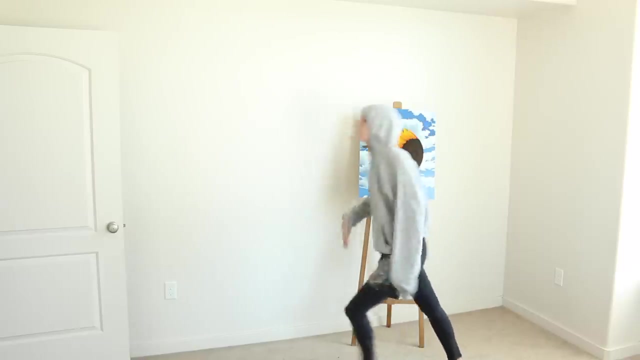 Combat this in one of three ways. One: leave the painting alone for a few minutes or a few days. When you walk back to it, you may see things you did not before. Two: get an outside opinion. Often a new person will be able to lend critique or advice from a new perspective. 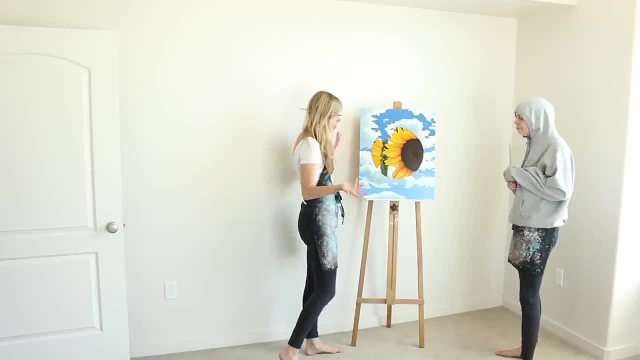 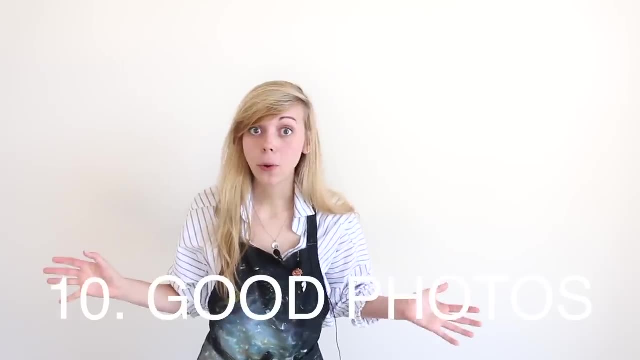 Three: photograph your work and look at it on your computer or compare it against your reference image. that same way, Seeing it in a new way, will shake up your perspective And give you fresh eyes. Ten photograph: well, So much can be done to elevate your work just through its treatment and final presentation. 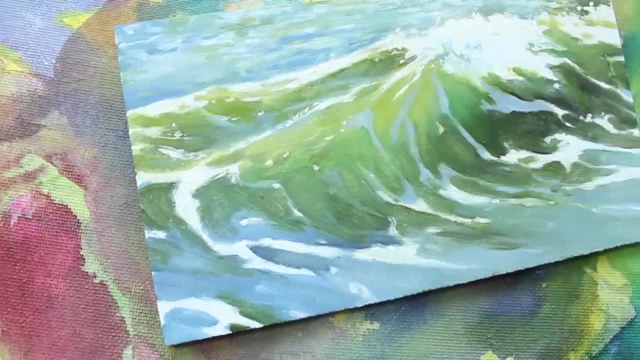 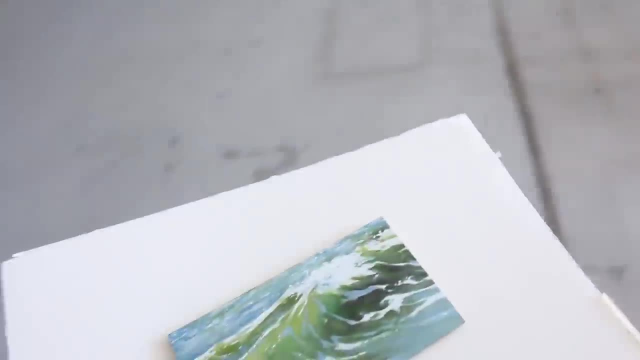 Do not diminish the quality of your work with a bad photograph. You can take something you might have seen as mediocre and increase or magnify its beauty by capturing it in a professional way. Have good lighting: Use natural daylight, outdoor shade, diffused light from an overcast day or daylight-coloured.